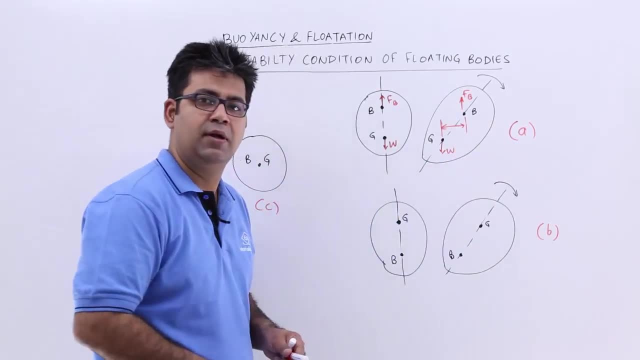 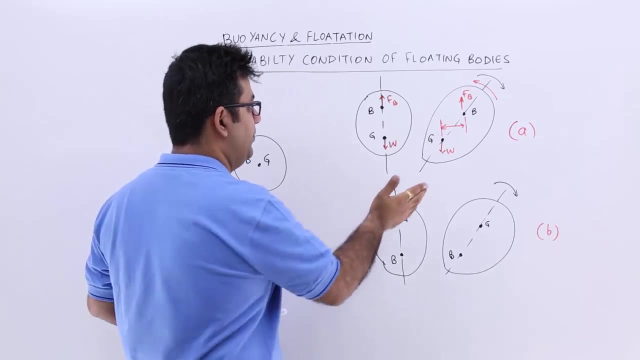 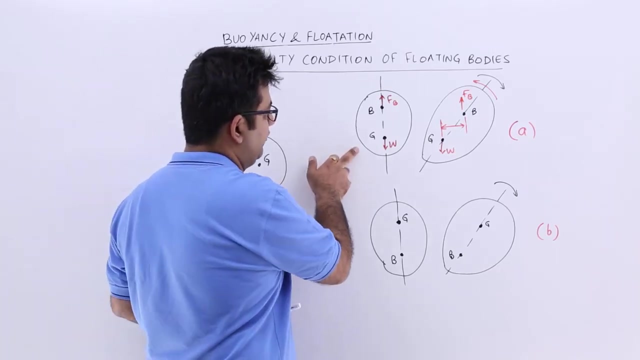 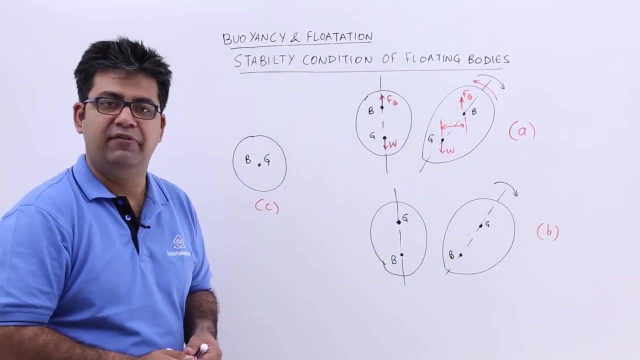 So this couple will create a moment, and the tendency of this moment is to turn this body in the anti-clockwise direction, Thus bringing the body back into the vertical position. So, when you have your center of gravity below the center of buoyancy, you will have a moment, with the help of this couple, which will turn the body in the opposite direction. 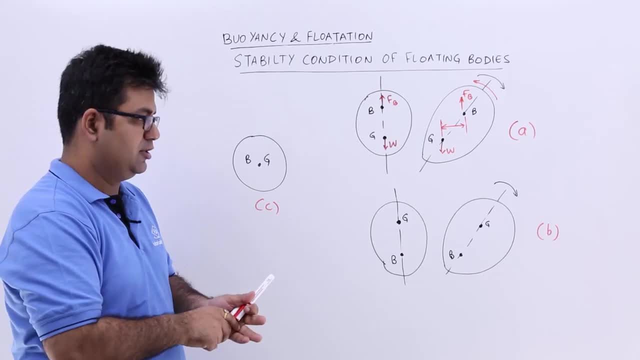 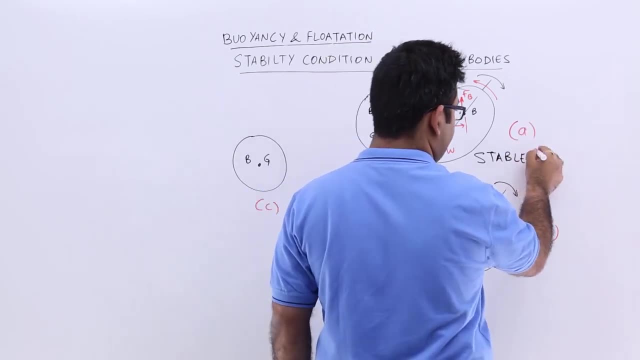 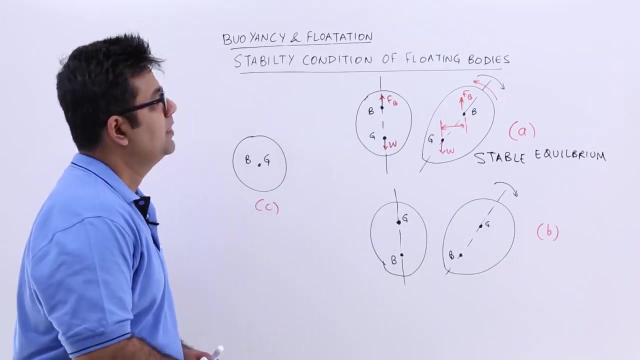 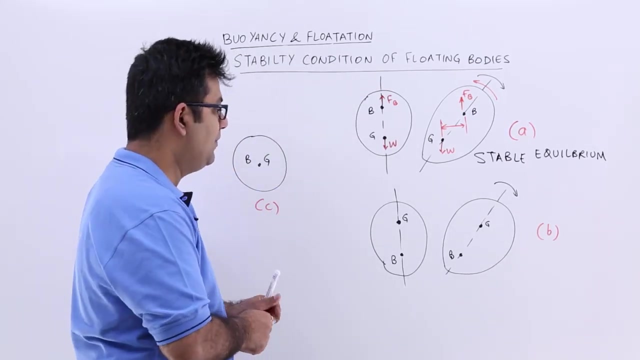 Thus bringing it back into the original position. So this kind of condition is called stable equilibrium. This is stable equilibrium Now if you come to this part where your center of gravity is above the center of buoyancy. So what happens at center of gravity? 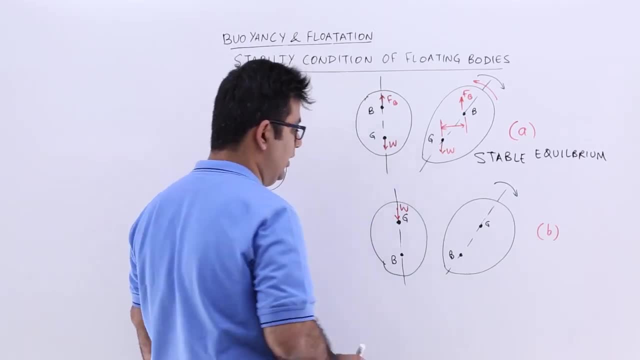 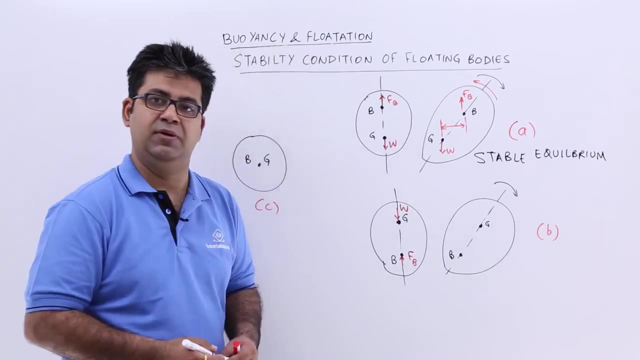 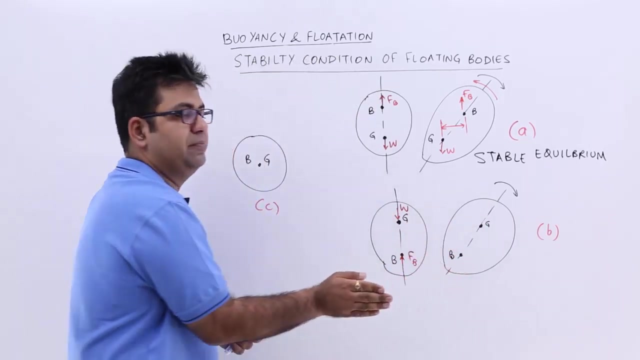 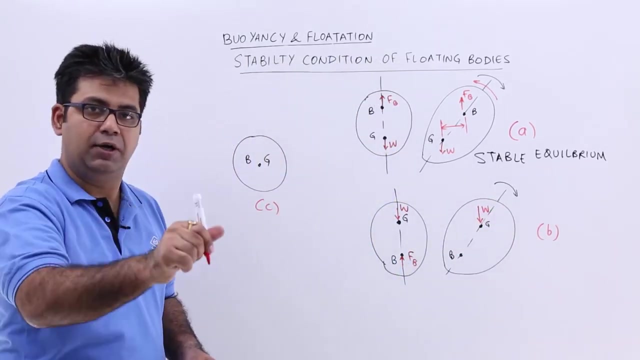 You have your weight acting vertically downwards. And what happens? at center of buoyancy, You have your buoyant force which is acting vertically upwards. Now, when you give it an angular displacement in the clockwise direction- this W- it is still acting in the vertically downwards direction. 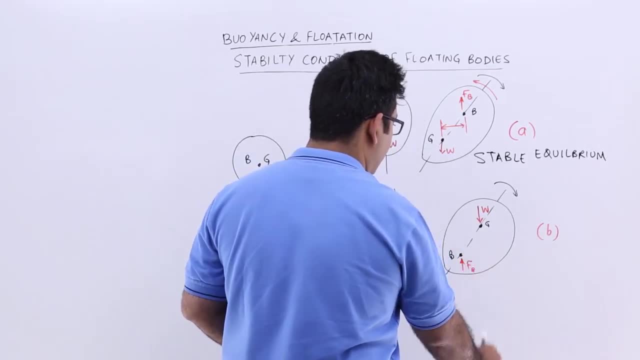 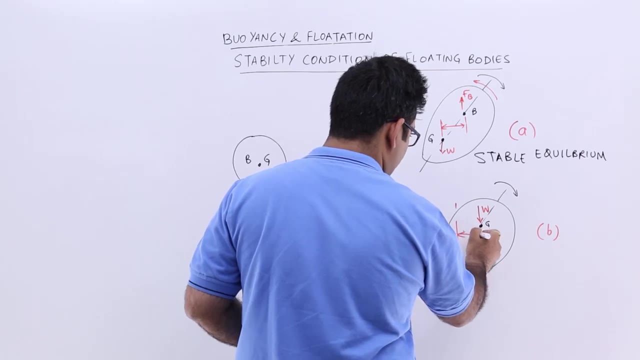 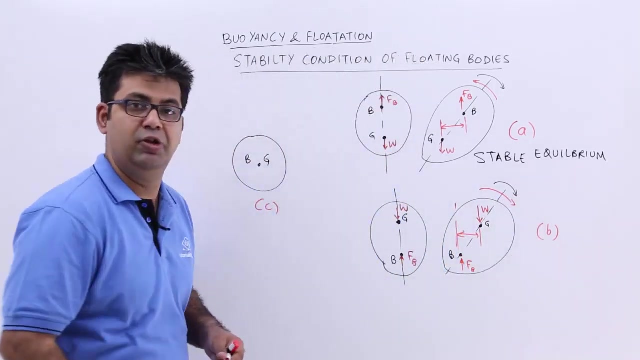 And this FB is still acting in the vertically upwards direction. So this again constitute a couple And the moment of this couple will produce a further rotation of the body in the same direction. So due to this couple, or due to the moment of this couple, 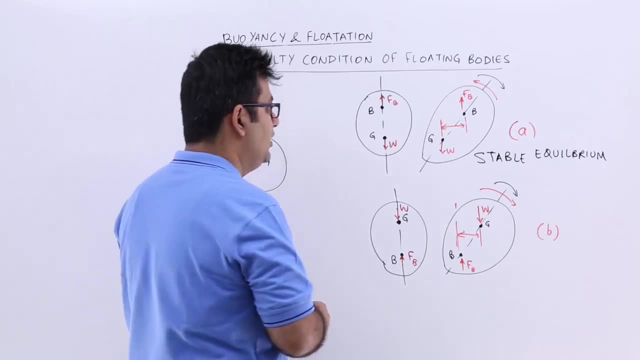 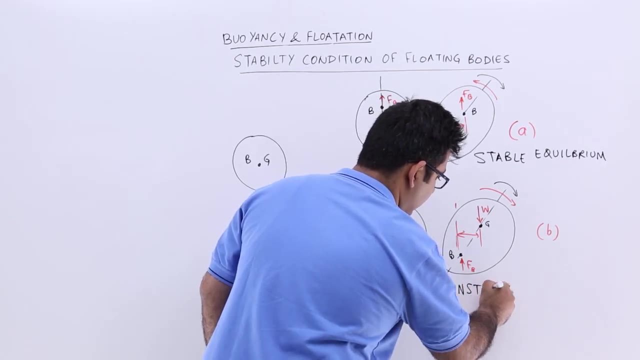 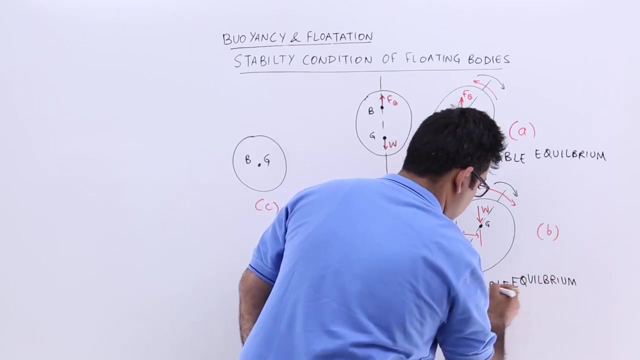 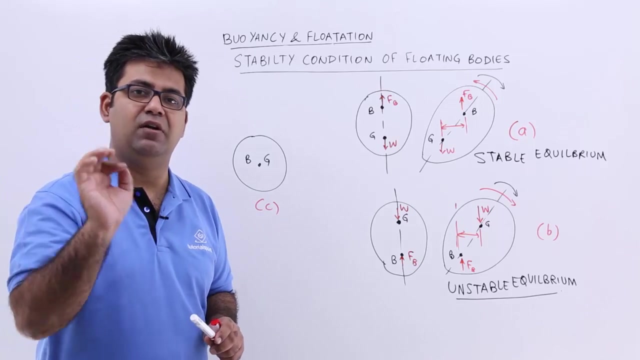 the body will not come back to its original configuration. Thus this kind of a condition is called unstable equilibrium. This is called unstable equilibrium. Now we come to the third figure, wherein your center of gravity, at the center of buoyancy, they are coinciding at one point. 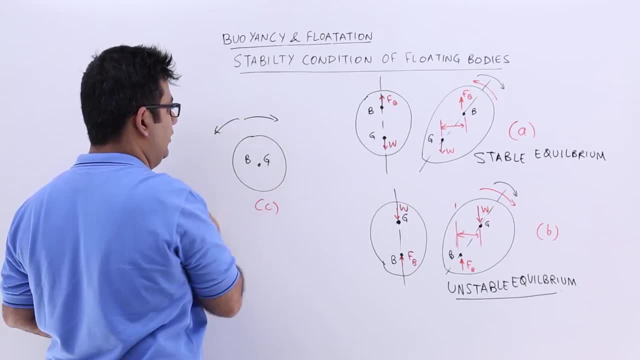 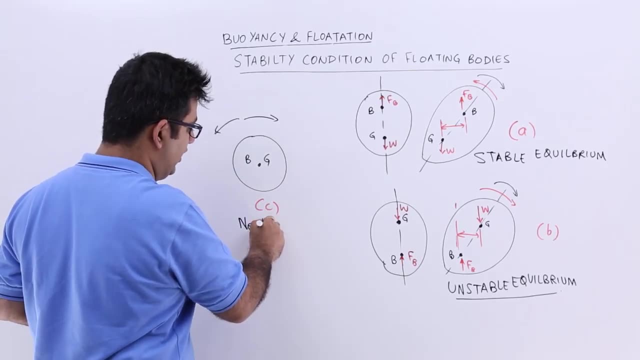 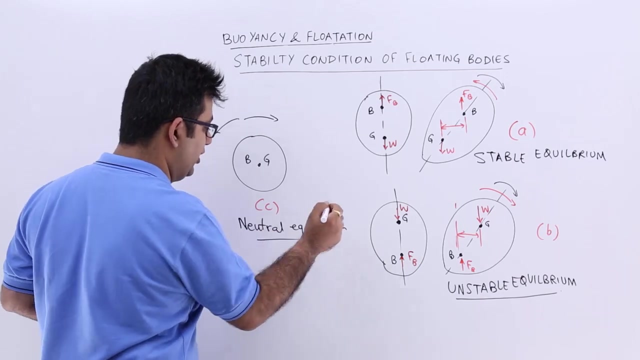 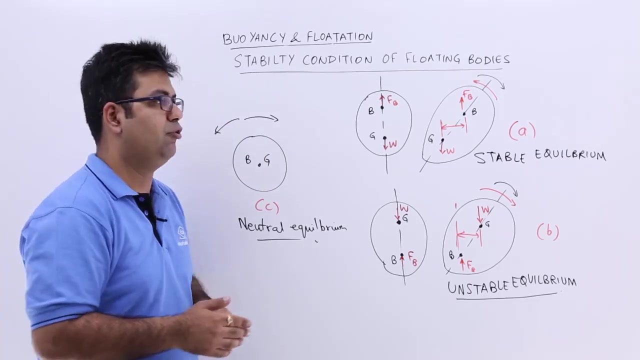 So you give it any displacement in any direction, this will stay as it is. So this is called neutral equilibrium, When your center of gravity and the center of buoyancy, they intersect. So these three are the stability conditions of floating bodies. I hope you got it.